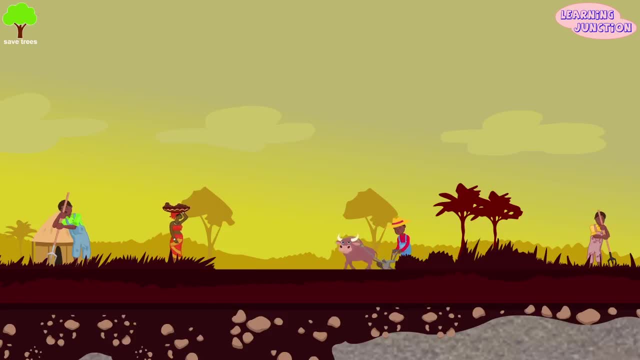 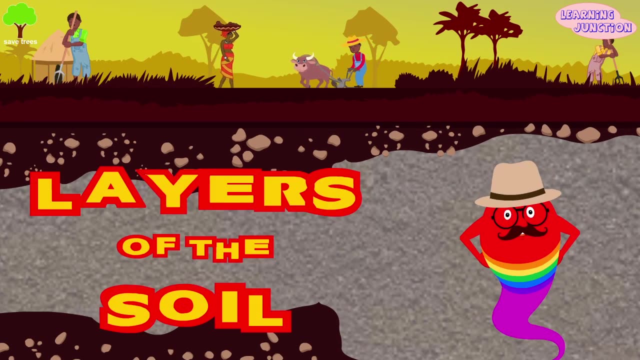 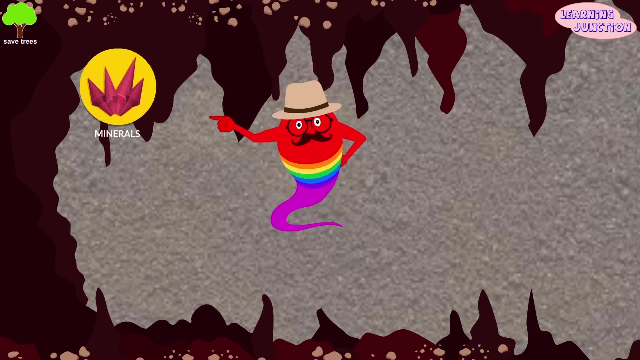 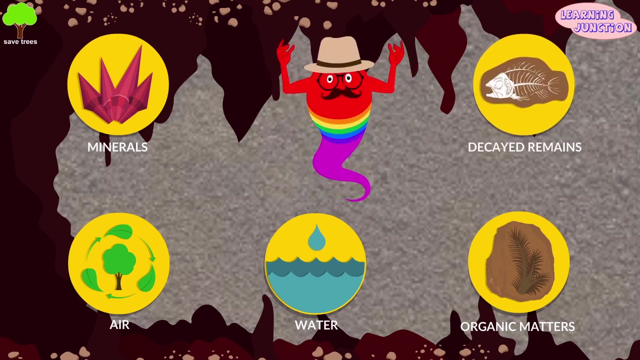 Hello friends, Today we'll learn about layers of the soil. Soils are complex mixtures of minerals, air, water, organic matter and various organisms that are the decaying remains of once-living things. Soil is made up of many layers, known as horizons. 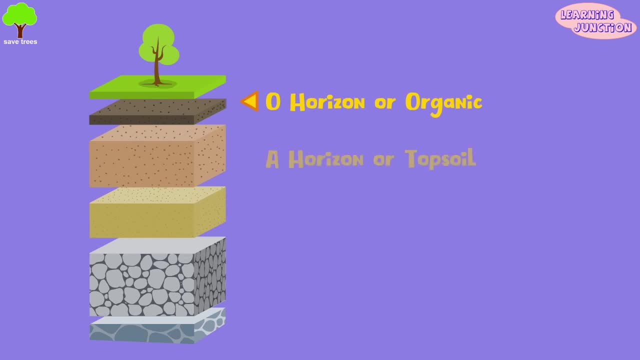 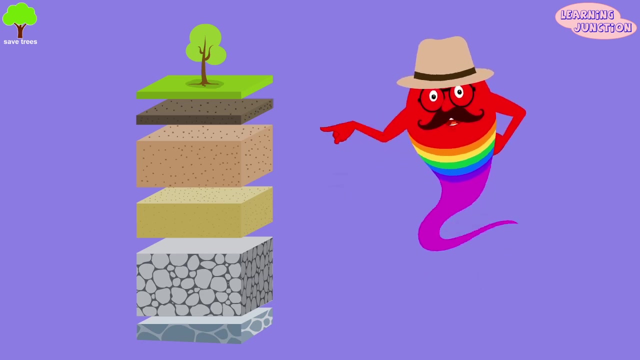 They are O-horizon, or organic A, or topsoil B, or subsoil C, or parent material, and R-horizon, or the bedrock. Each layer has its own characteristics that make it different from the other layers. 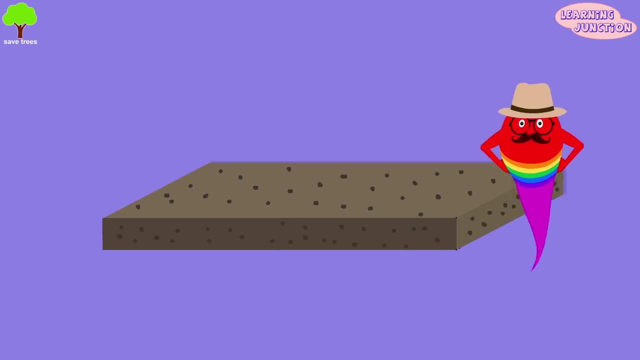 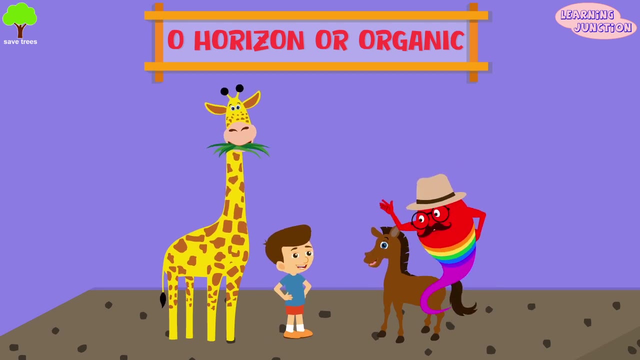 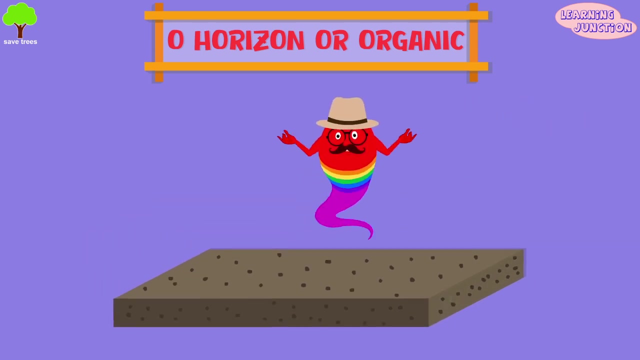 Let's learn about each layer one by one. O-organic: This is the top layer where we all stand. Oh, hello friend. This is a layer of organic matter and is approximately two inches thick. This is made up of living and decomposed materials like leaves, plants and bugs. 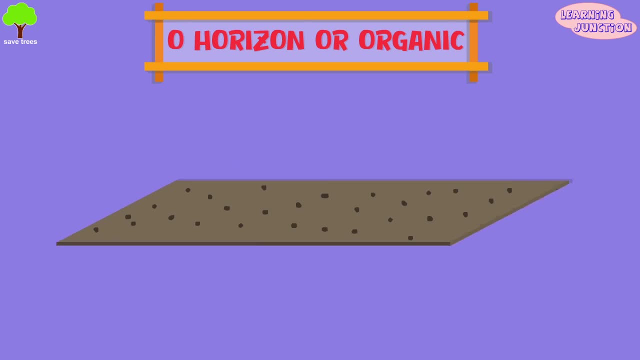 Sometimes this layer is very thick or thin or may be absent. A-topsoil: This layer consists of organic matter and decomposed materials. The humus, or compost, makes the topsoil dark, brown, porous and soft to hold enough water and air. 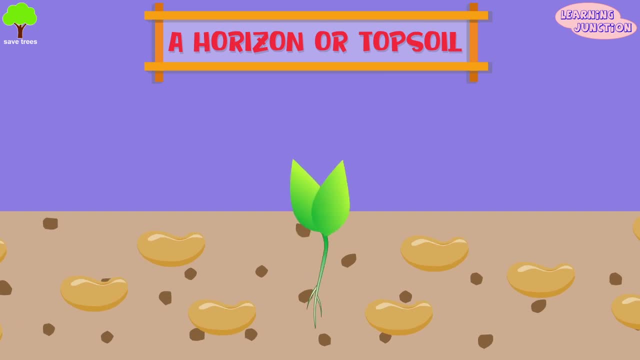 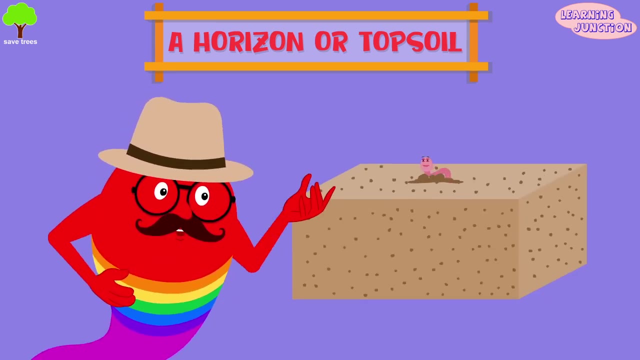 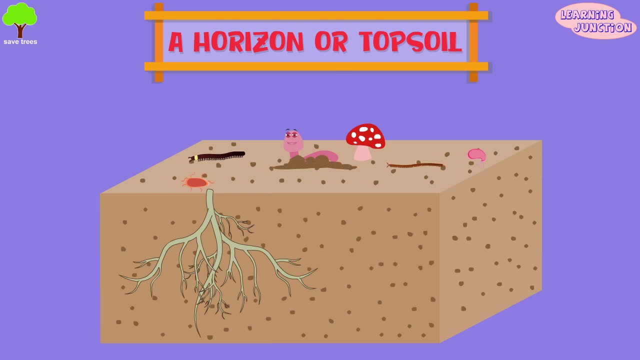 That's why in this layer, the seeds germinate and roots of the plants grow. Oh hey, Mr Earthworm, you look great. Guys see many living organisms like earthworms, millipedes and centipedes. 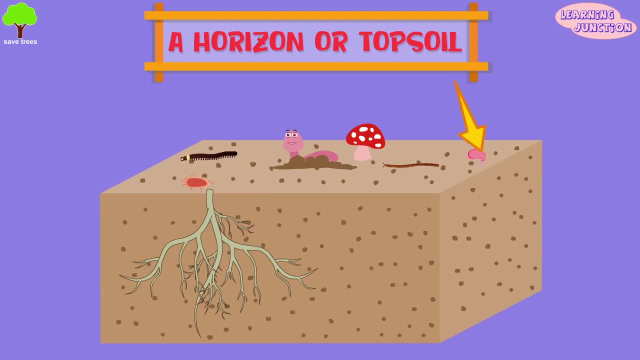 are made up of organic matter. This is a layer where we all stand. Oh, hello friend, This is a layer where we all stand. Guys see many living organisms like earthworms, millipedes and centipedes, bacteria and fungi. 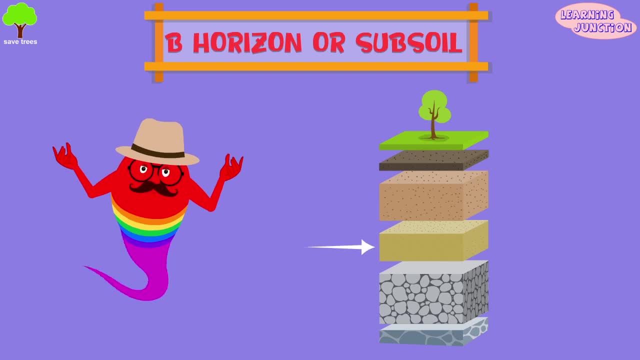 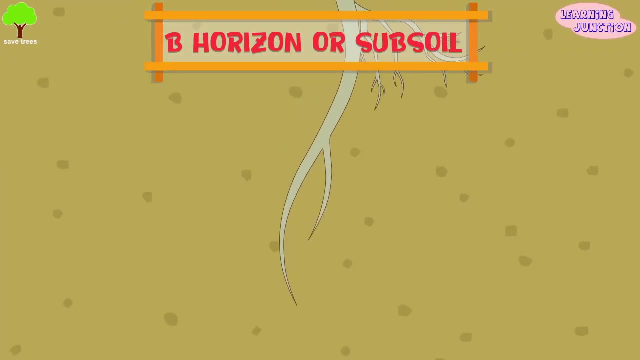 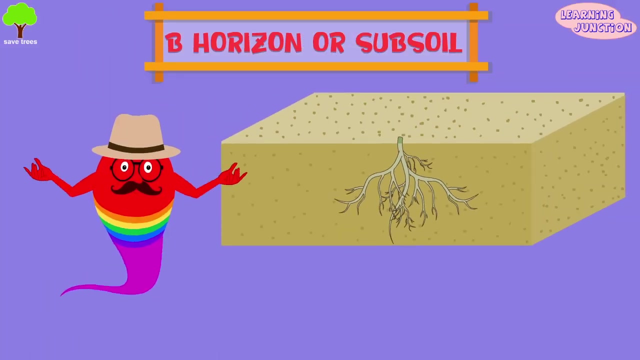 are found in this layer of soil, B-subsoil. Just below the topsoil lies the other layer, called subsoil. It is comparatively solid and tighter than topsoil, so only large plant roots can reach here. It is lighter in color because there is less humus in this layer.